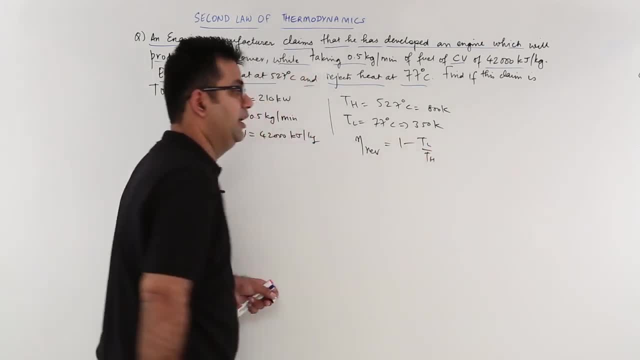 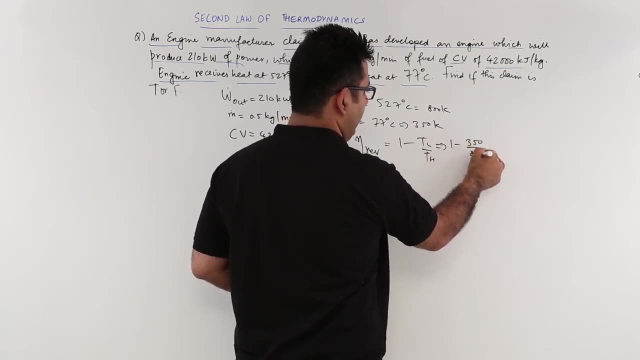 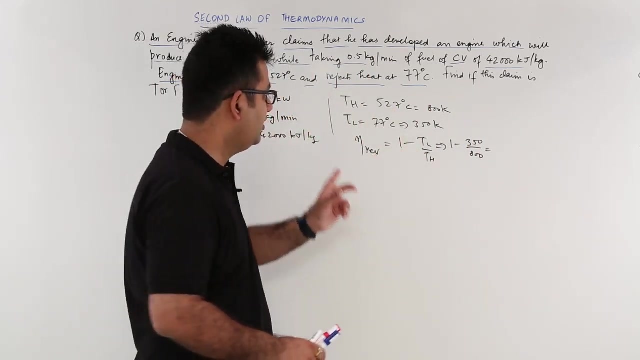 So reversible heat engine is 1 by TL, by TH. So when you put in the values so you had 1 minus 350.. Upon 800.. Remember this: never put in the values of temperature in degree Celsius, Always convert them into Kelvin and then only put the values because these are absolute temperature values. 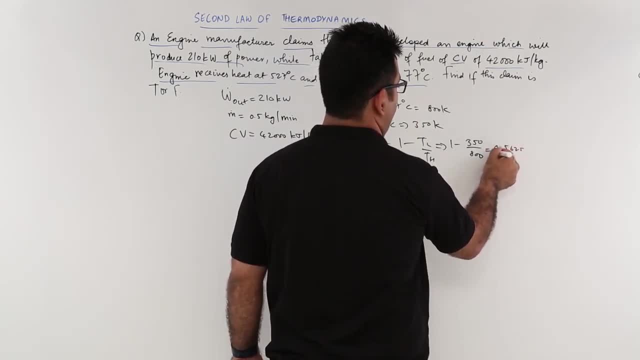 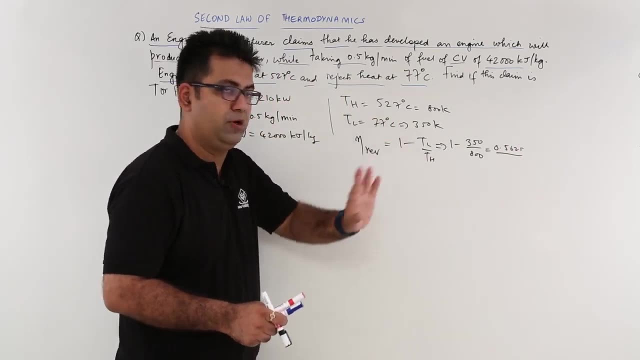 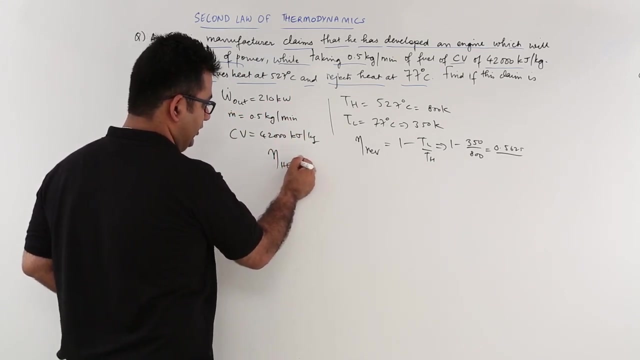 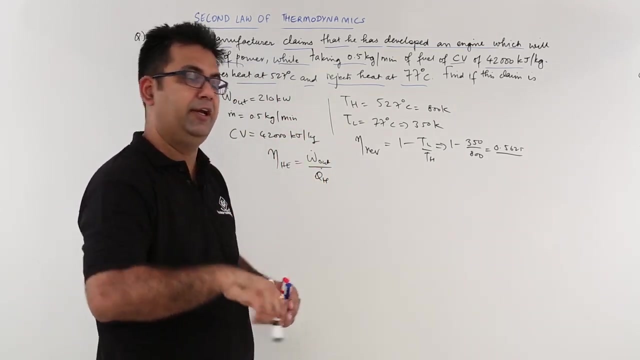 So this comes about to be approximately 0.5625.. So around 56% is the efficiency of a reversible heat engine which is working under these two temperature limits. Okay, now for an actual heat engine he has developed. this would be equal to: upon the rate of work output, upon the rate of heat. 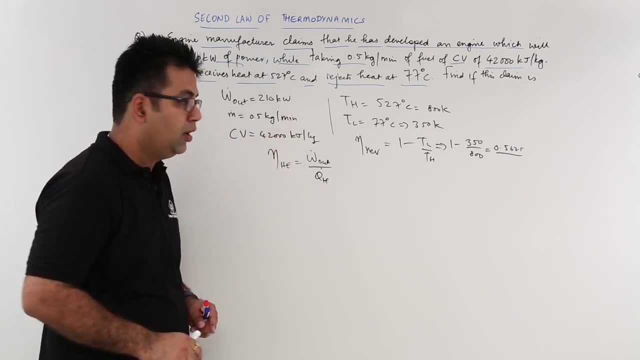 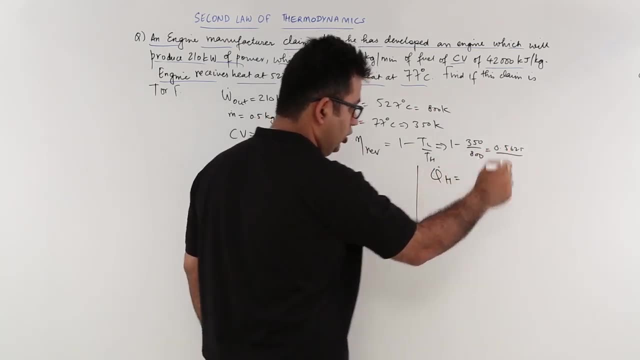 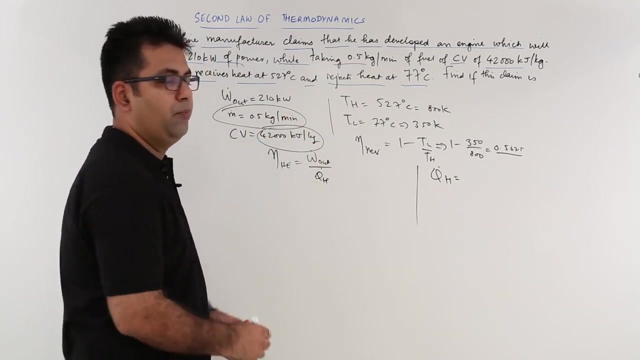 input. now work output, we know, is 210 kilowatts. what is the rate of heat input? let's find that out now. the rate of heat input, that is q h dot. you have calorific value of 42000 kilo joule per kg and you have a mass flow rate of 0.5 kg per minute. so that would give. 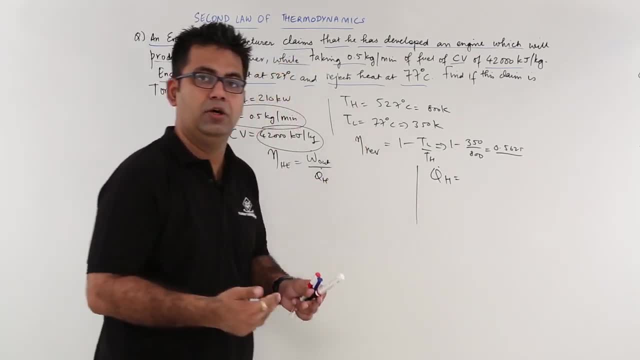 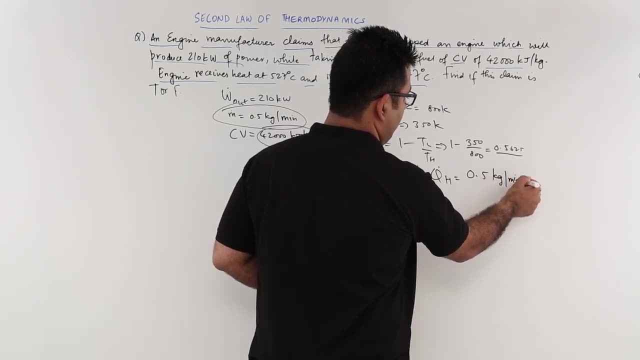 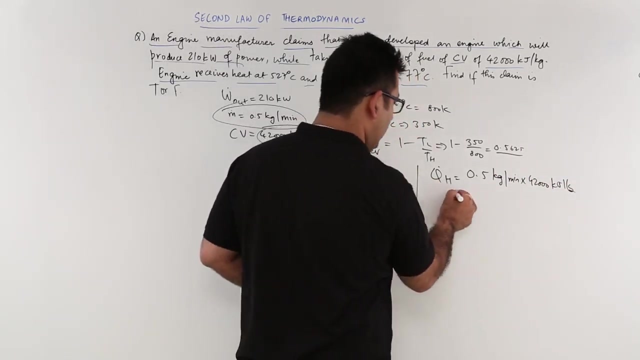 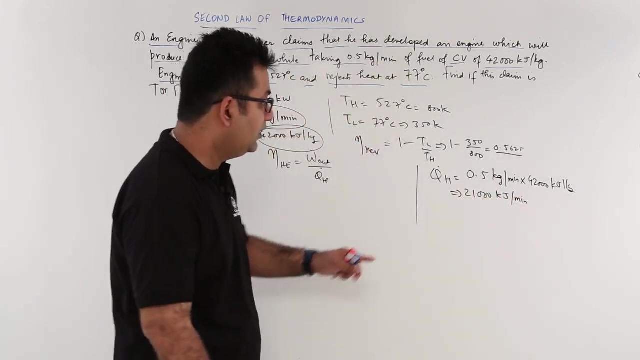 you kilo joule per minute or the heat flow rate you know into the engine, so that would give you 0.5 kg per minute. into 42000 kilo joule per kg, alright, that gives you 21000. that's the half of 42 kilo joule per minute. if you convert this into kilowatts, that is. 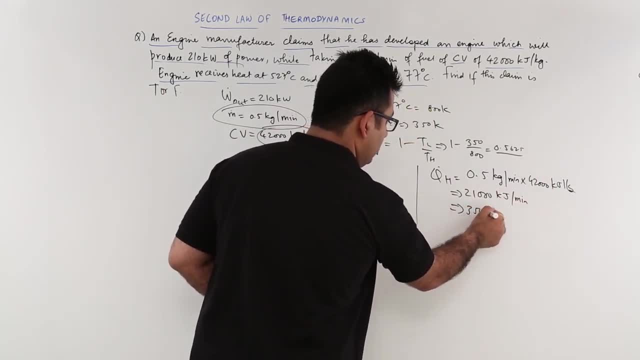 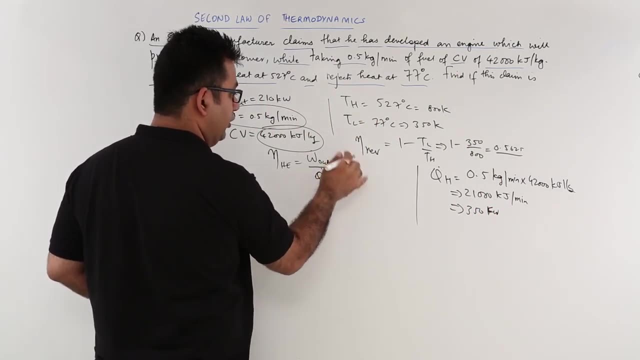 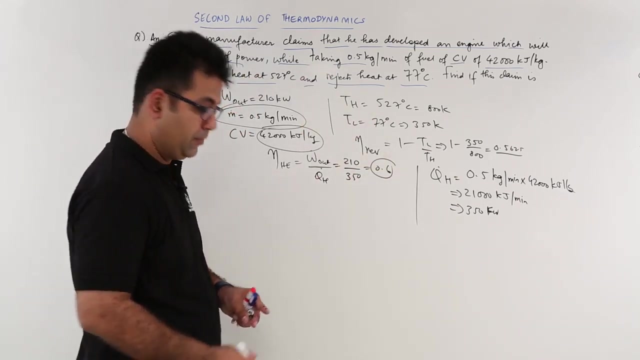 kilo joule per second. this would translate into kilo joule per minute, 350 kilowatts. okay, now you can use it here, because you need to have the same units. so this is 210 upon 350, which is 0.6, 60% if you compare these two efficiencies, that is for. 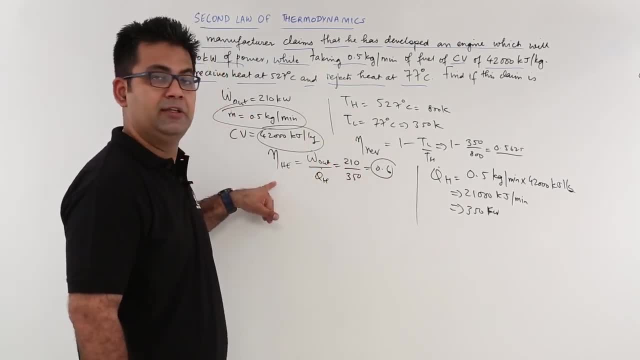 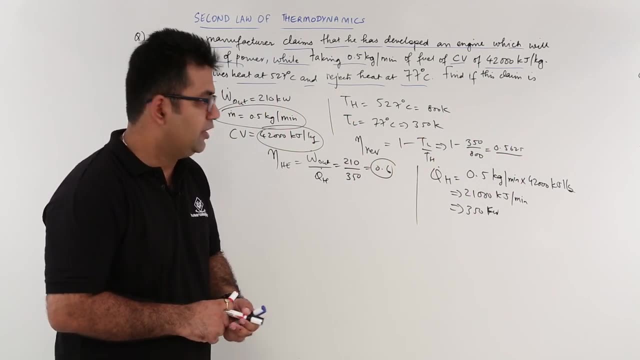 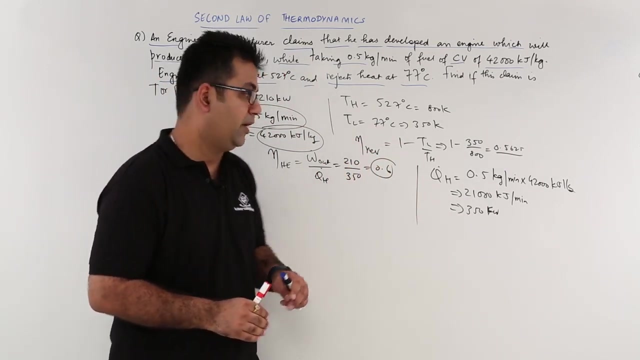 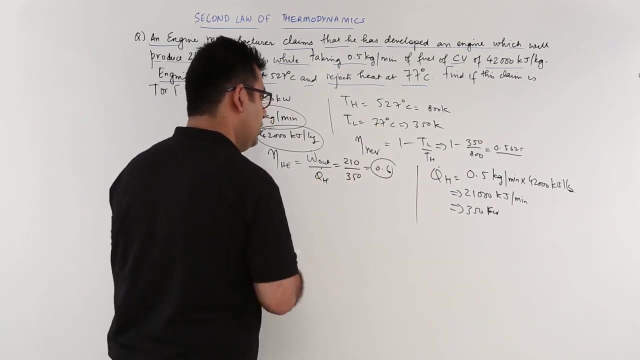 the reversible engine and for the actual heat engine these values are not valid. why? because in every situation, always, the reversible engine has the highest possible efficiency, but in this case you have the reversible efficiency as a lower values compared to the actual values. so you have this condition, which is not possible.